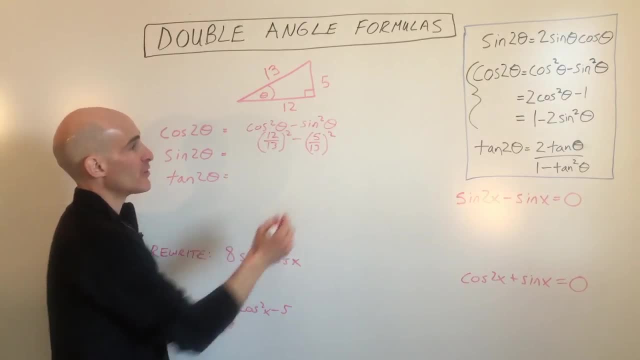 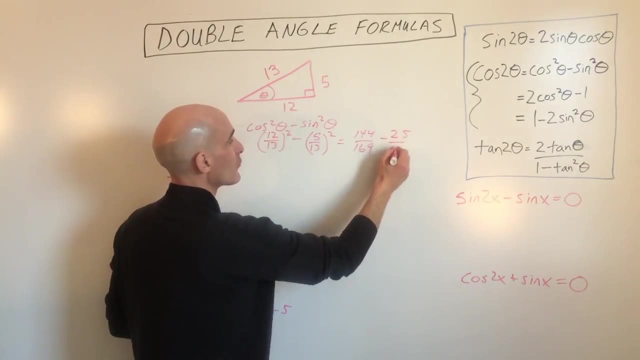 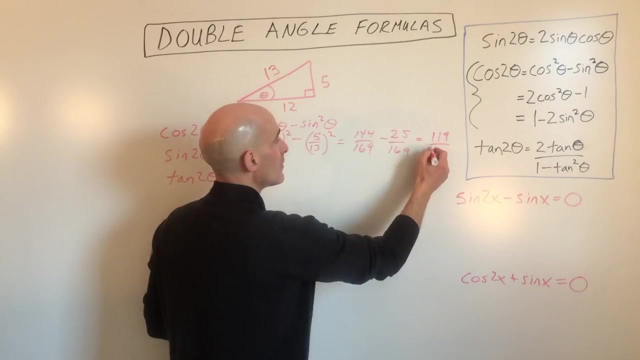 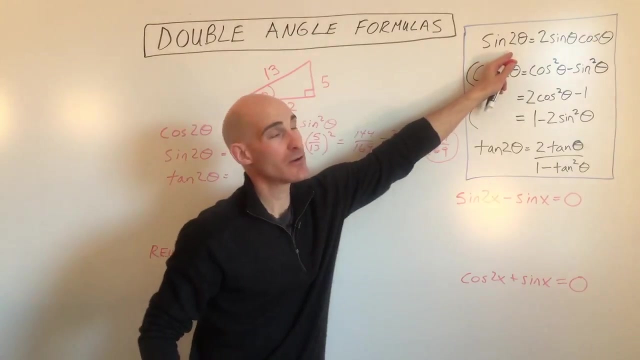 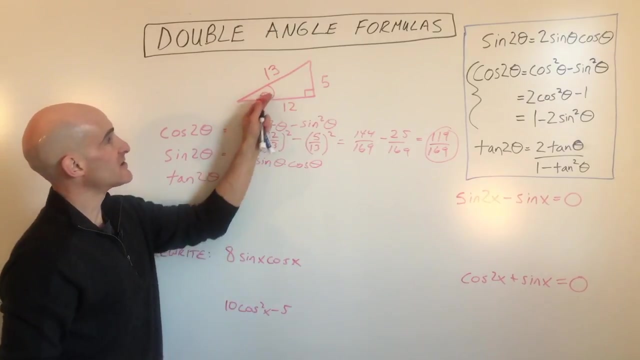 squared and if we simplify that, we get 144 over 169 minus 25 over 169, which equals 119 over 169.. Okay, so that's an exact answer. Sine of 2 theta- we're gonna use this top one here, so we have 2 sine theta times the cosine of theta. Sine is: 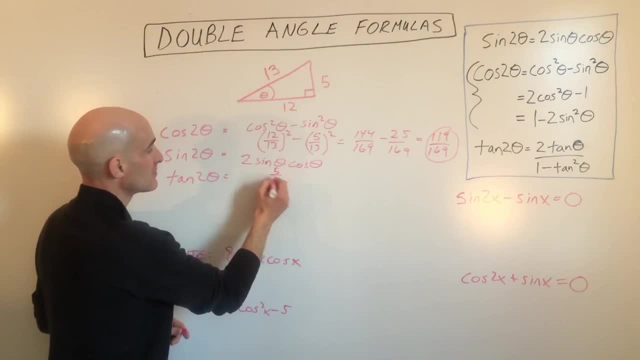 opposite over hypotenuse. so that's 5, 13 times 2, which is 2 over 1.. Cosine theta, which is adjacent over hypotenuse, that's 12- 13, and then all we have to do is multiply across. that gives us 60, 120 over. 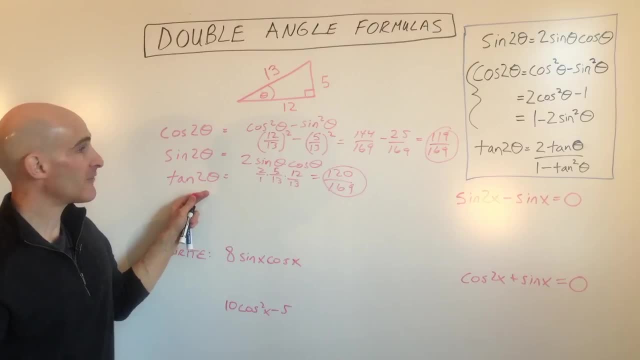 169.. Okay now, if we want to find out tangent of 2 theta, we have a couple of choices. We can use the tangent formula here, or we can take sine divided by cosine, and so tangent of 2 theta is the same as Sine over cosine. sine of 2 theta. 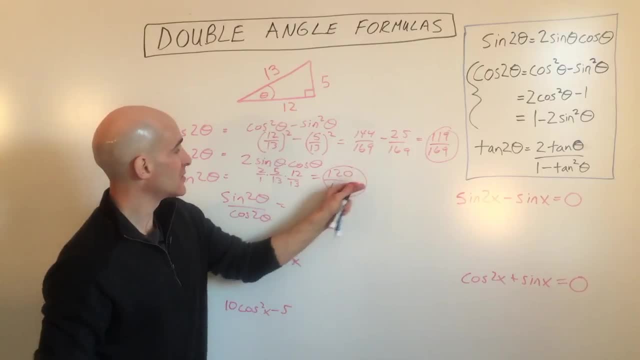 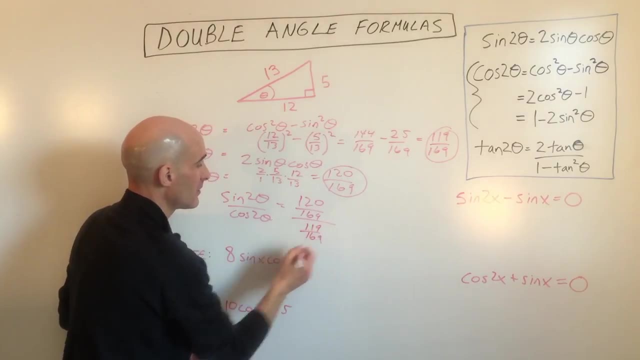 over cosine of 2 theta. So if we do that that's going to be a, a Cobalt E farking table. 4 di pancakes, 8 waffles, 120 divided by 119, and you can see if we multiply the numerator and denominator by: 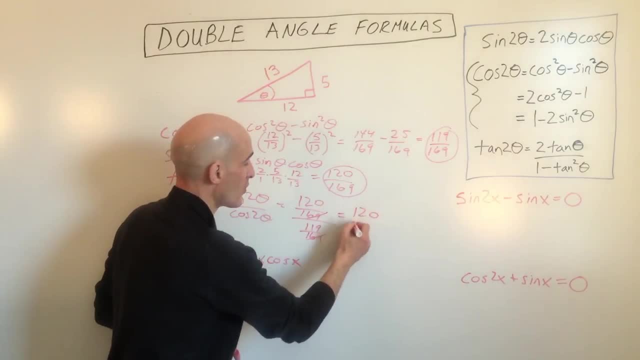 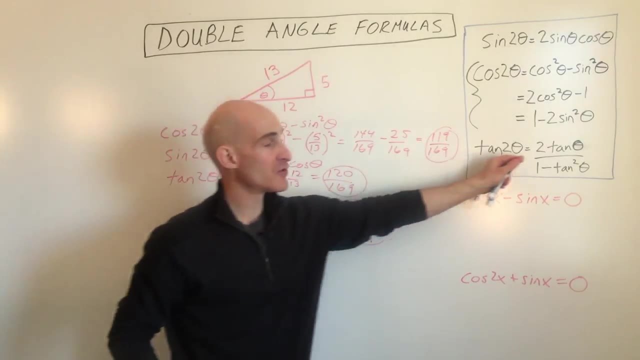 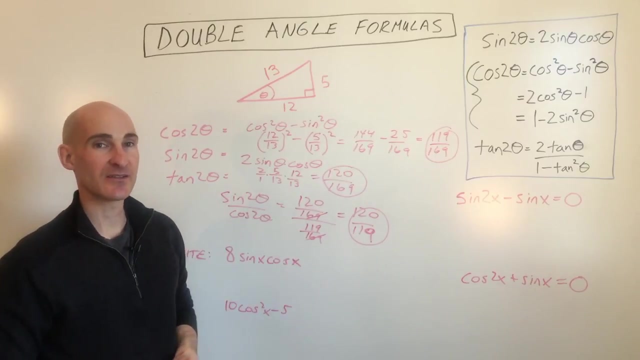 169,. we're just going to end up with 120 over 119.. So if you want to double check your work, you might want to do the tangent double angle formula and just verify that you're getting the same result. If not, you can go back and check the sine and the cosine. Okay, now the next ones. 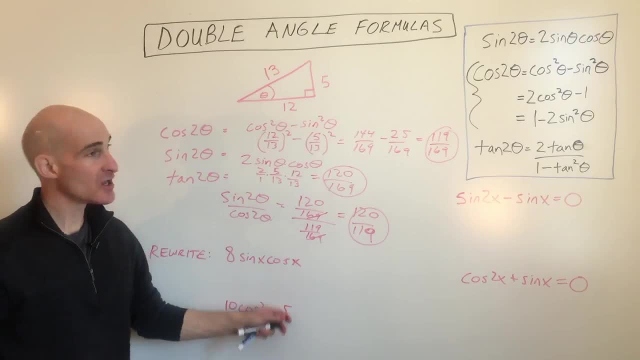 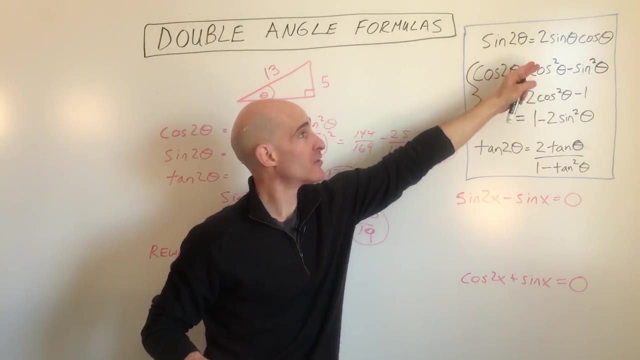 we're going to take a look at are how to rewrite some of these expressions using the double angle formula. So what's happening here? again, just focusing on the fact that these are identities, they're identical the left and the right sides. If they give us something that looks like the 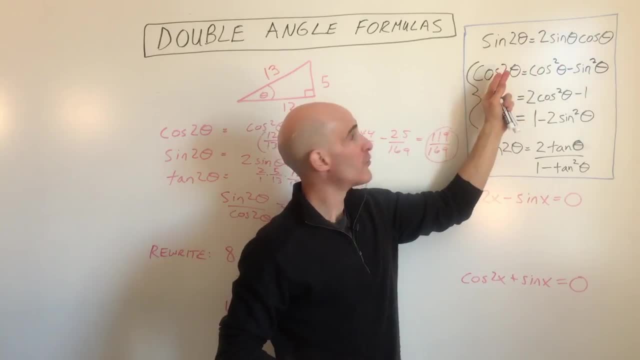 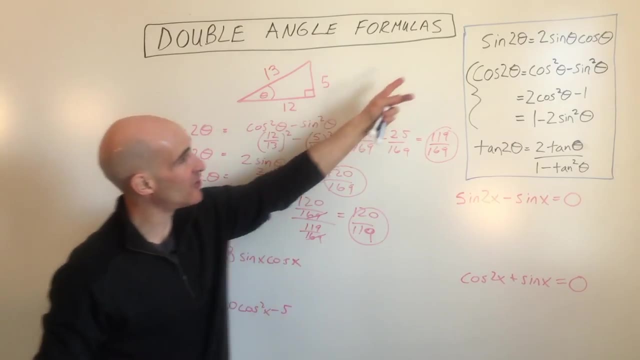 right side. we can rewrite it okay in terms of the left side. So what we're going to do here is look at this formula: 8, sine x, cosine x. Which one does that look like? It looks like the top one right. So what we're going to do 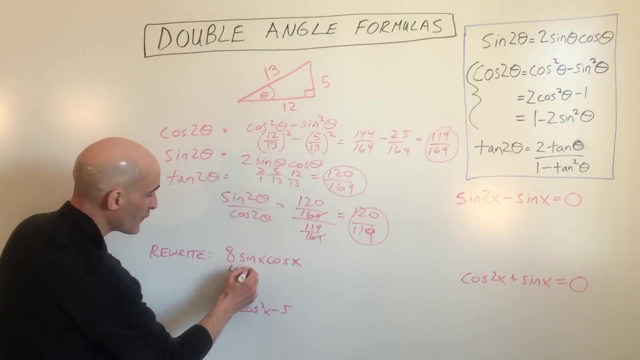 is we're going to say: well, this isn't exactly like that. but if we factor out a 4, 4 times 2 is 8.. And so now we have 2 sine x, cosine x, which is the same as sine of 2x times this 4.. 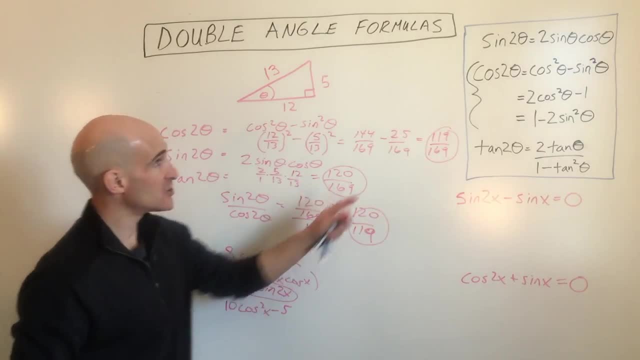 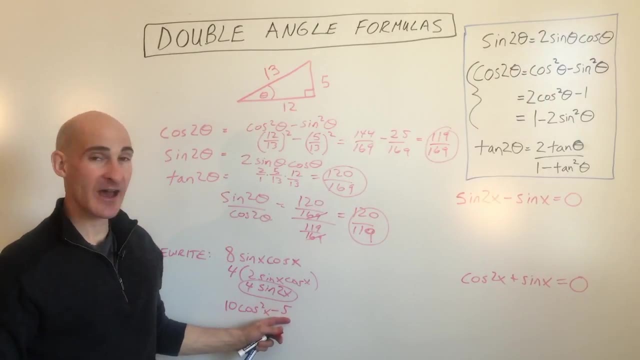 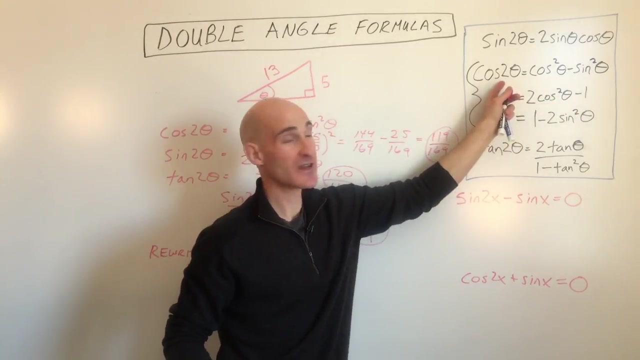 So there you go. We've just rewritten the expression, using a double angle instead of a single angle. We went from the right side to the left side. Okay, this next one: 10 cosine squared x minus 5.. Which one does that look like? That one looks like this one here in the middle. This is a cosine. 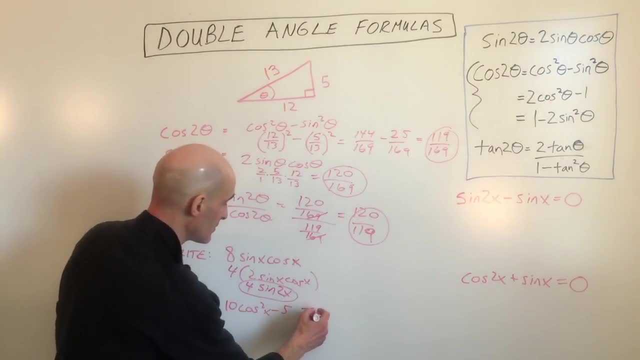 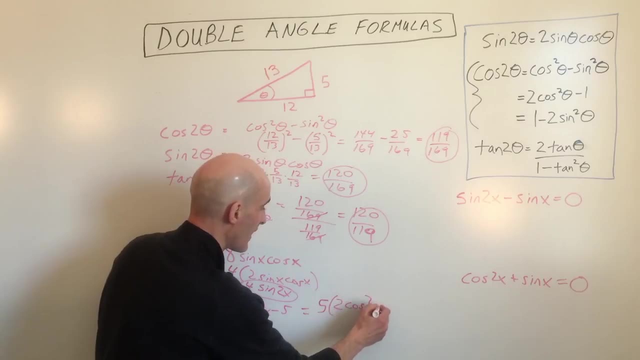 double angle formula. So what we have here is we're going to factor out a, 5. So that's 2 cosine squared x minus 1, okay, And we know, 2 cosine squared x minus 1 is cosine of 2x. So this is: 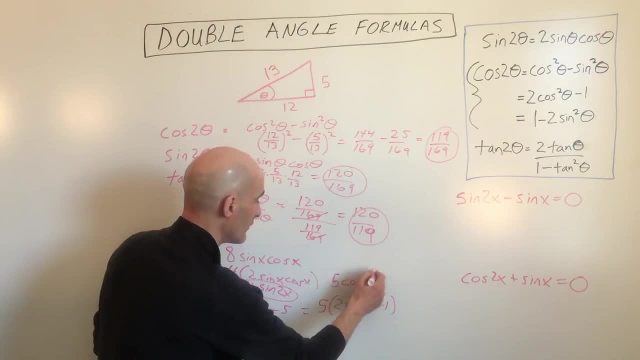 just going to be 5 times the cosine of 2x. Okay, so they're right. So we're going to do that. Okay, so they're right, So we're going to do that. So we're going to do that. So we're going to do that. 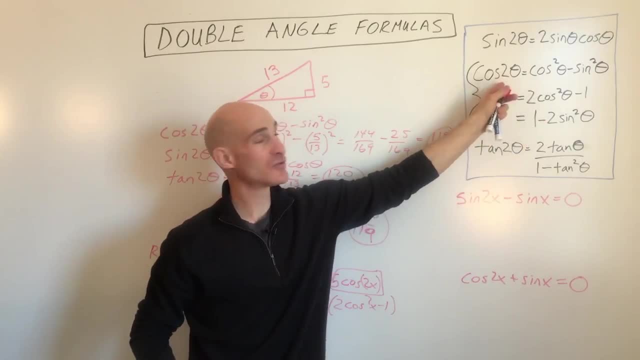 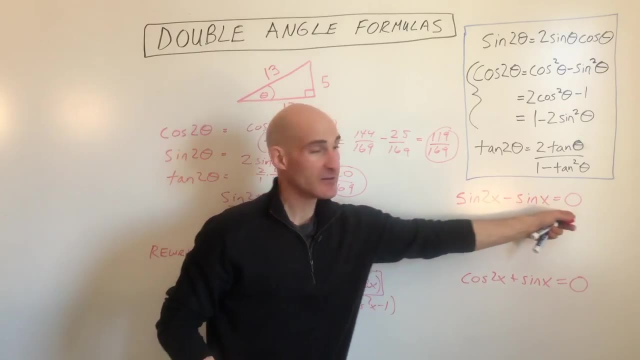 Again, we're just going from the right side to the left side, going from a single angle to a double angle using the identities. Okay, these last two examples I want to show you. we're going to be solving trig equations. You can see there's a double angle in here as well as a single angle. 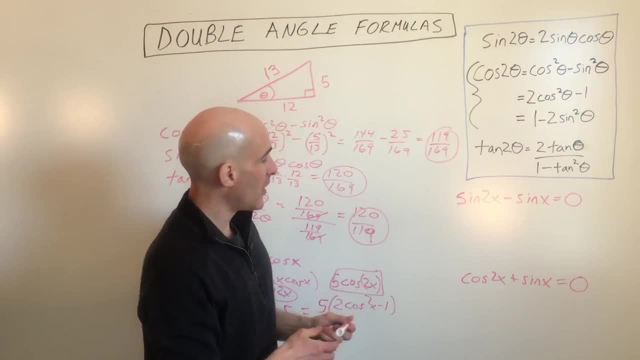 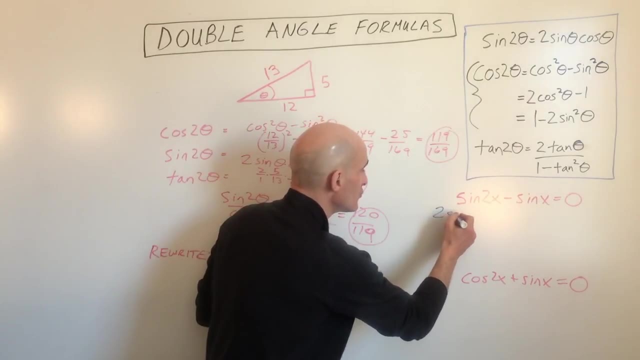 So how can we work with that? Well, for this one, why don't we use our double angle formula, expand it out? So this is going to be 2 sine x, cosine x Minus sine x. Okay, that's the sine x. And then what we can do is we can factor and set the factors. 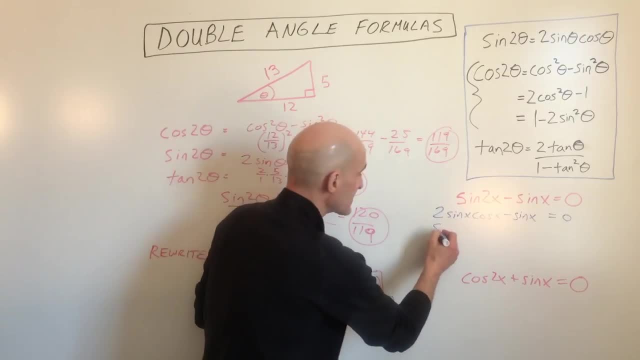 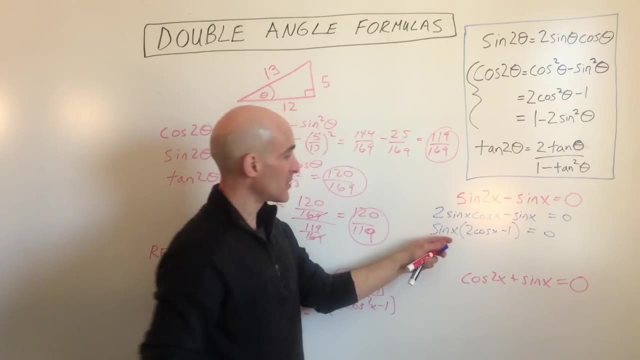 equal to 0. So I'm just going to factor out a sine, because that's in common in both groups. So sine of x equals 2 cosine x minus 1.. And then what we can do is we can set each group equal to 0.. So this: 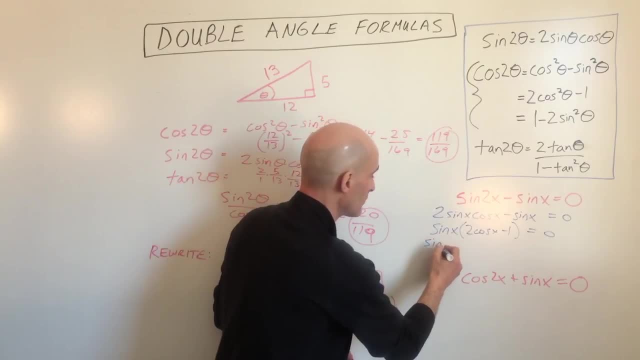 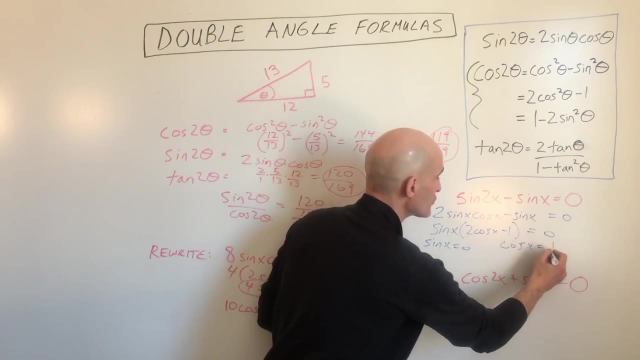 is going to give us sine of x equals 0. And if we set this one to 0, we're going to get cosine x equals 1 half, Cosine x equals 1 half. And then what we're going to do is we're going to set each group. 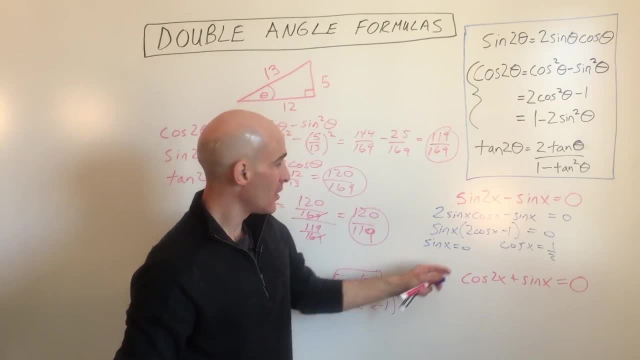 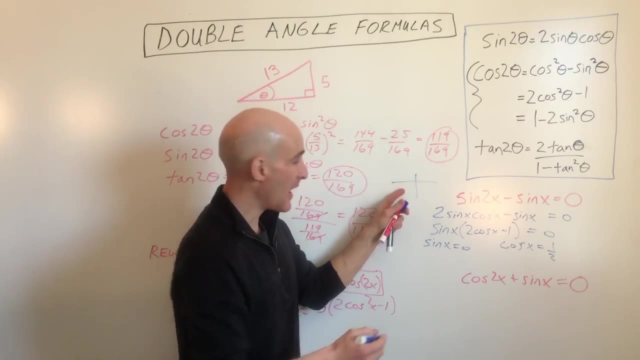 equal to 0. So sine of x equals 1 half. We're just adding the 1 and dividing by 2.. So now we go to our unit circle. Where does sine equal 0?? Sine equals 0 over here at 0 and pi. Okay, so 0, pi. And where? 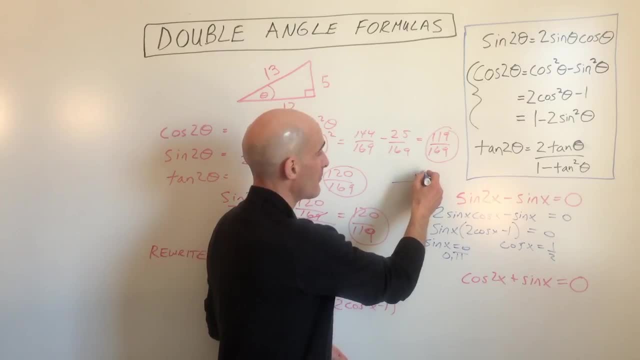 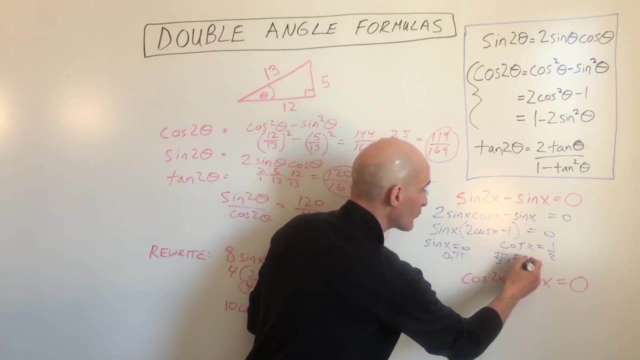 does cosine equal a half? Cosine equals a half here at pi over 3 and 5 pi over 3.. And if you need help with that, go back to my video on the unit circle and review that. But if you really know, 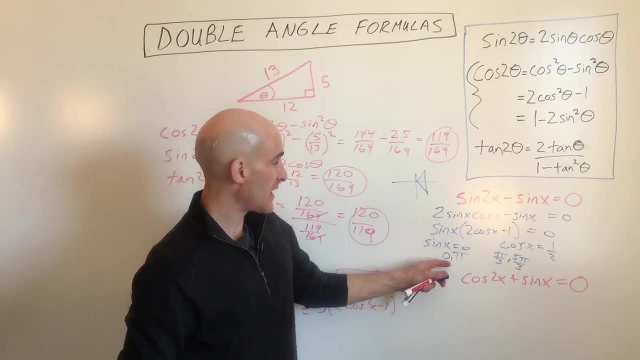 your unit circle really well, you'll be able to find these angles. So that's that one. It's 0, pi pi over 3, and 5 pi over 3.. That's just from 0 to 2 pi once around the unit circle. 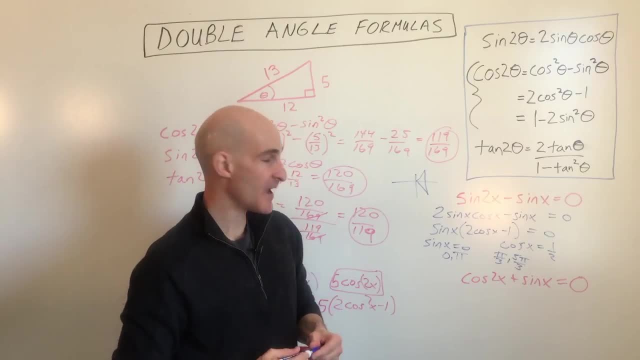 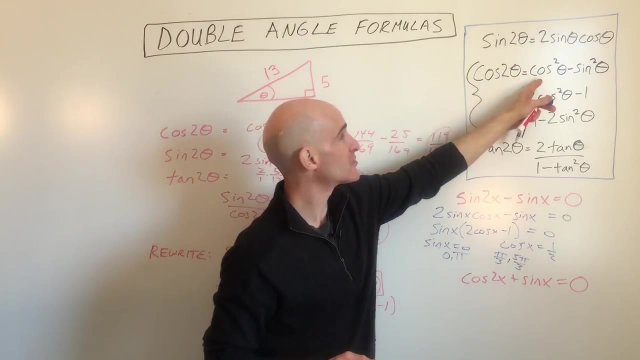 Okay, in the last example, cosine 2x plus sine x, we're going to use the cosine double angle formula. But here's the question: Which one should we use? Should we use the first one, the second one, the third one? Well, it doesn't really matter, But if you make a good decision, it'll make the 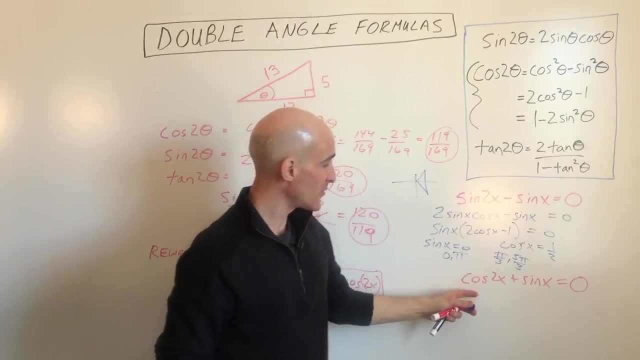 work a little bit easier. Let's go with this bottom one. This way, we can get everything in terms of sines. See how. this is cosine 2x and this is sine 2x. This is cosine 2x. This is cosine 2x. 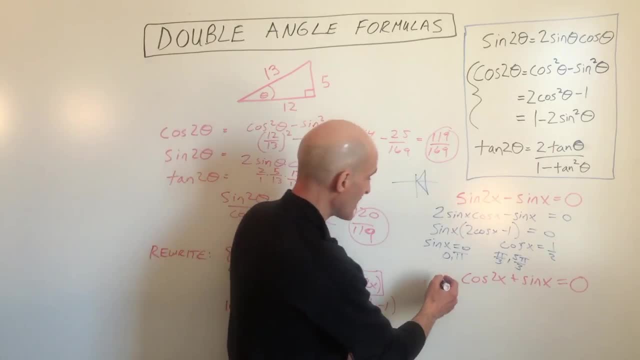 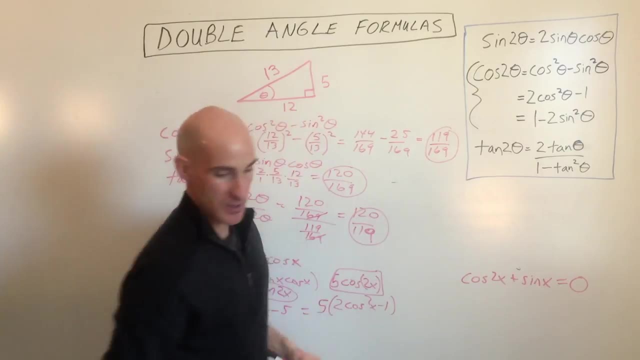 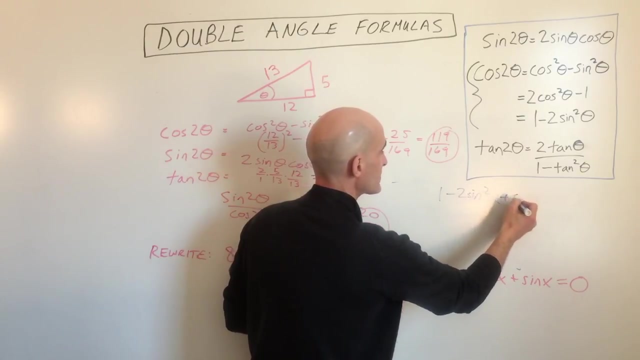 We're going to get this cosine 2x in terms of sine. So that's going to be- let's give ourselves a little bit more room here- So that's going to be: 1 minus 2 sine. squared x plus sine x equals 0.. 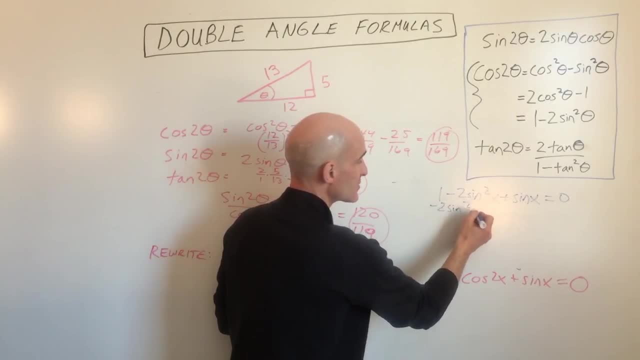 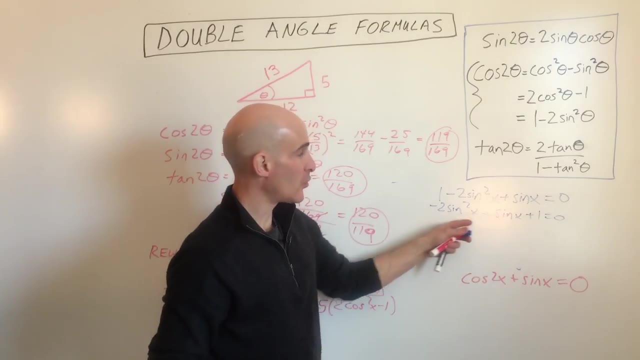 I'm going to write this in descending order: Negative 2 sine squared x plus sine x plus 1 equals 0.. This is a trinomial, It's a quadratic form, And what we're going to do is we're going to factor. 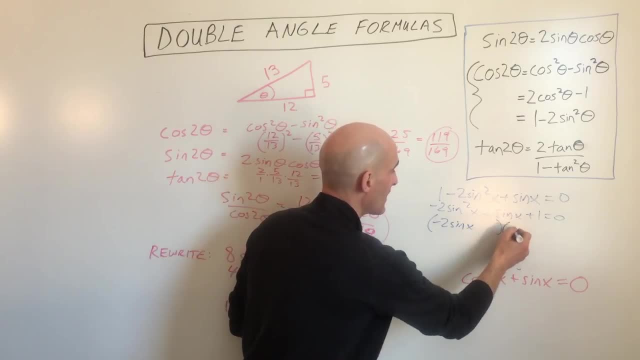 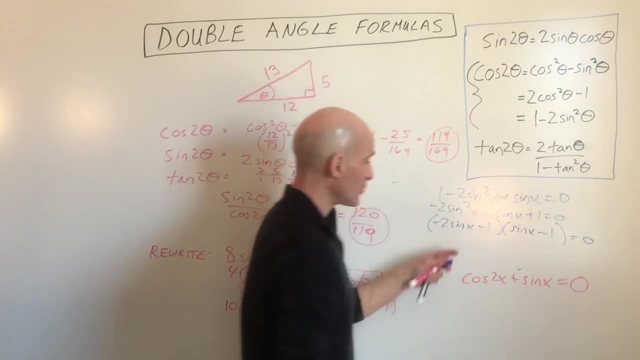 it So negative 2 sine x and positive sine x, And we've got negative 1 and negative 1.. So that factors. And then what we do? we set each group to 0. So we get sine equals 1 and we get. 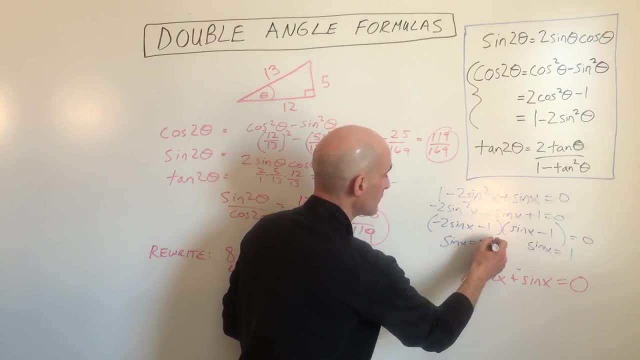 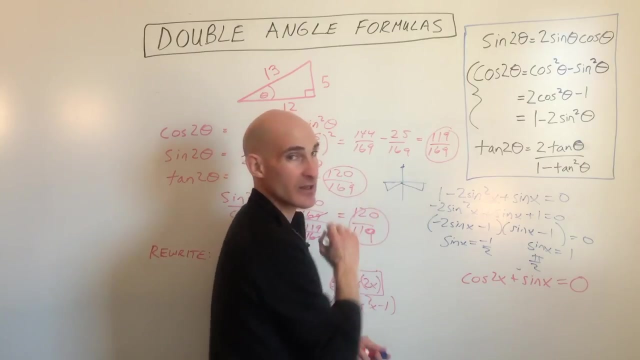 sine equals negative 1 half. Okay now, where does sine equal negative 1 half and 1?? Well, we know sine is 1 here at pi over 2.. And we know sine equals negative 1 half in the third and fourth quadrants, at 7 pi over 6 and 11 pi over 6..